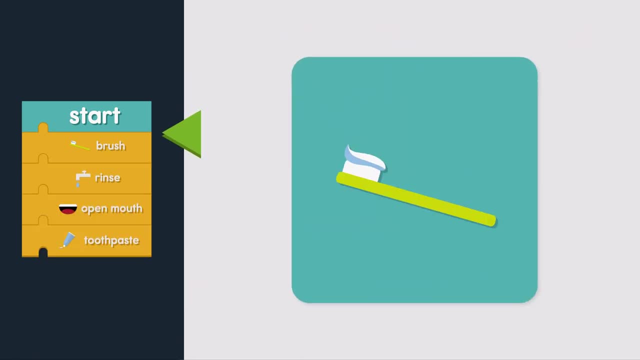 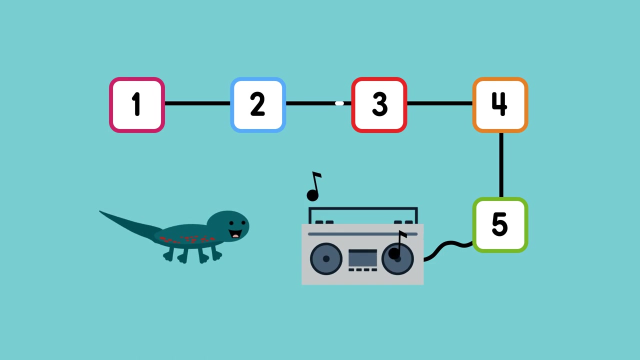 Alright, I can do this: Brush, rinse open mouth. put toothpaste on, Put toothpaste on, rinse, brush open mouth. Put toothpaste on open mouth, brush, Brush, rinse. You gotta say the right steps from the start until it's done. If you don't, it won't work and that's no fun. 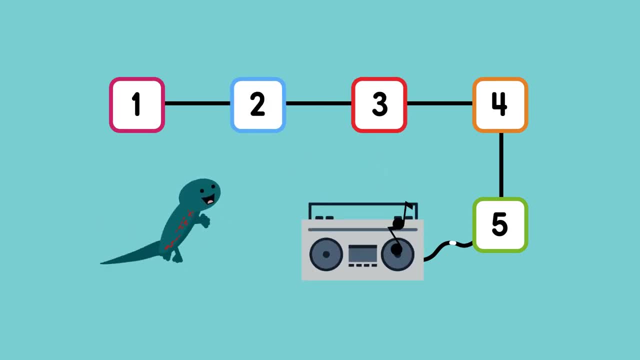 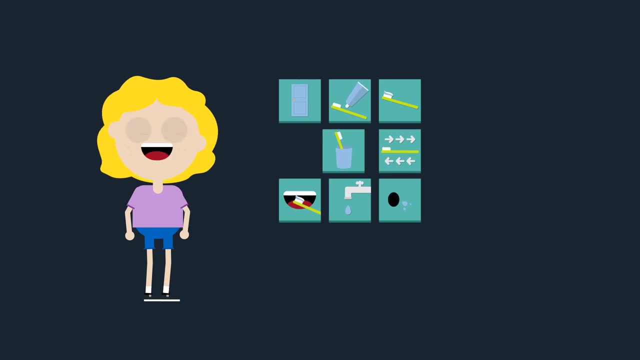 It's called sequencing and it's the order of things. It's how we gotta talk. when we talk to machines, You know what? Let's get way more specific. Many other steps actually go with it. To brush your teeth proper, gotta know what to do. 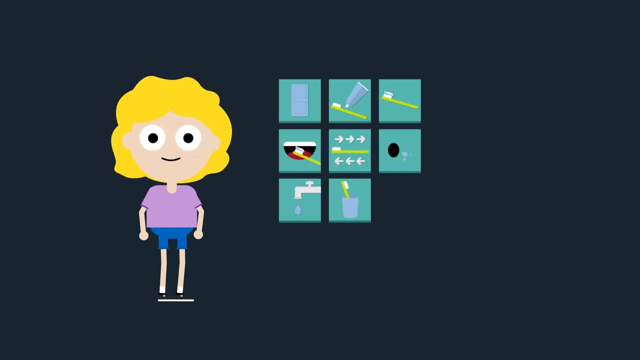 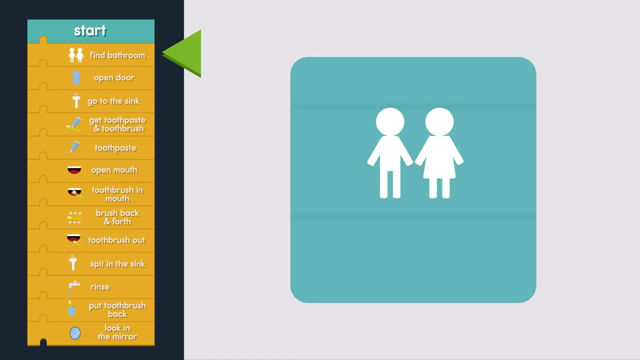 Let's go step by step until it is through. Okay, give it a try. Be real specific for me now. First you Find the bathroom, Then you Open the door, Then you Go to the sink, Then you Get your toothbrush and the toothpaste. 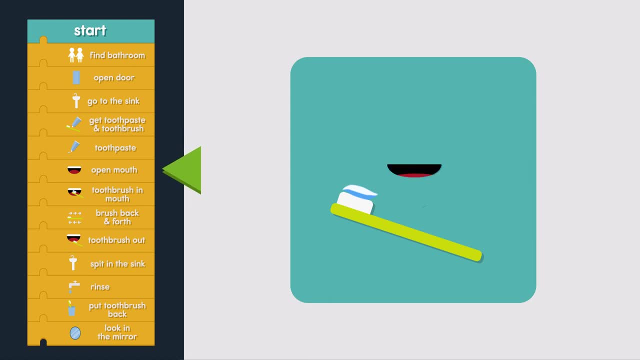 Then you Put the toothpaste on the toothbrush, Then you Open your mouth, Then you Put the toothbrush in your mouth, Then you Brush back and forth, Then you Take the toothbrush out, Then you Spit in the sink. 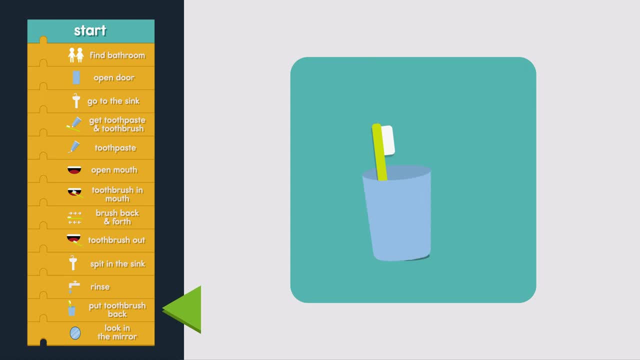 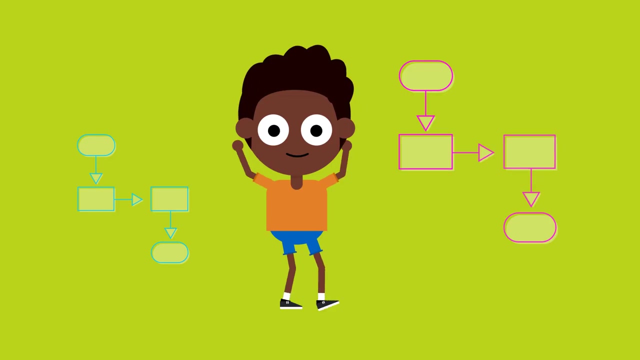 Then you Rinse your mouth and the toothbrush. Then you Put the toothbrush back. Then you Look at your clean teeth in the mirror and smile and say you are the best toothbrusher ever. Wow, that's a lot of steps. There are so many. 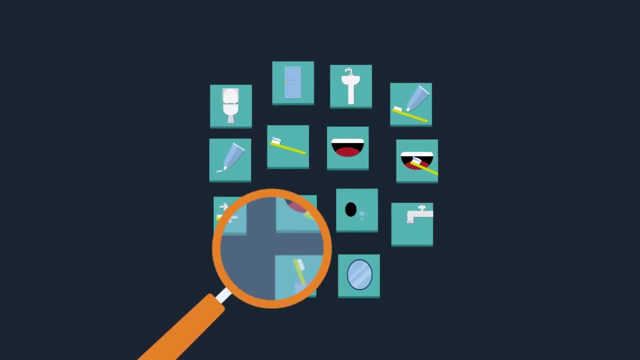 Double check to make sure you didn't miss any. Gotta tell the computer exactly what to do, Cause if the sequence isn't right it won't work for you. You gotta say the right steps From the start until it's done. 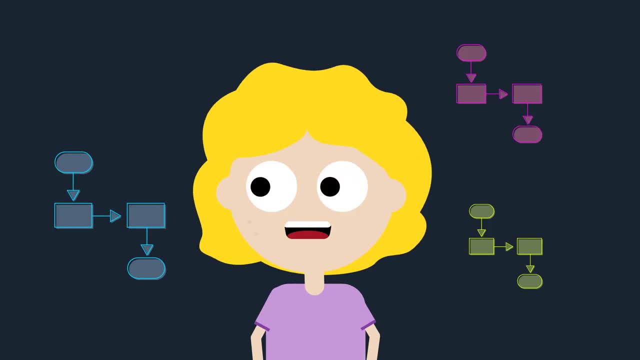 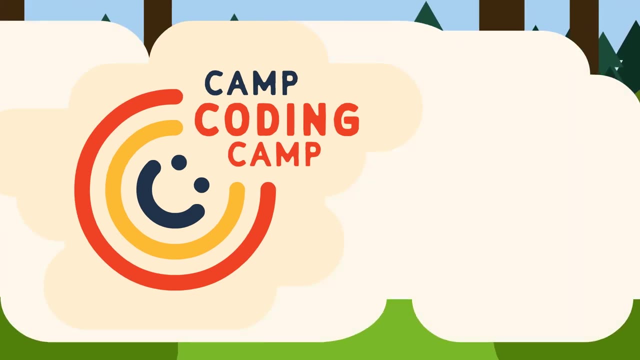 If you don't, it won't work and that's no fun. It's called sequencing and it's the order of things. It's how we gotta talk when we talk to machines. So, speaking of sequencing, what are we gonna learn about next? 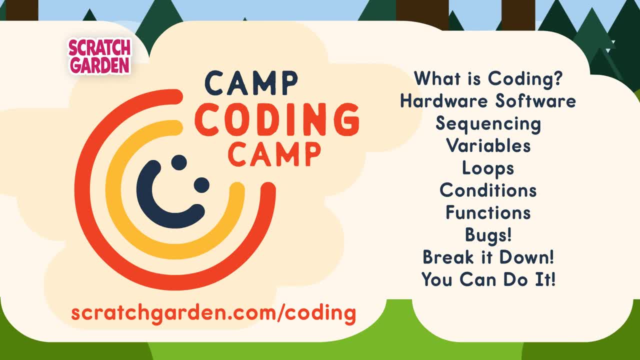 Variables- Yes, variables, I love vari-. wait, what are variables Variables, To see what's going on when it's not perfect or something. What are variables Variables? We're gonna do that in a second. Variables: What are variables?